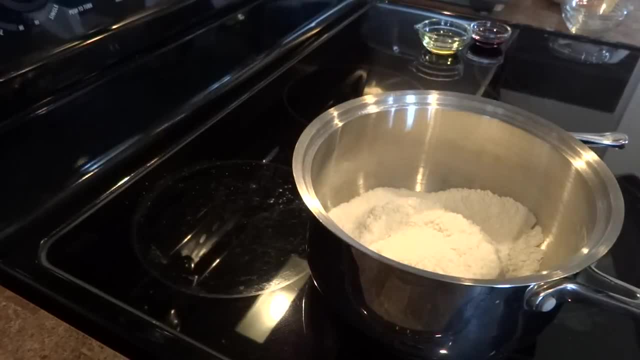 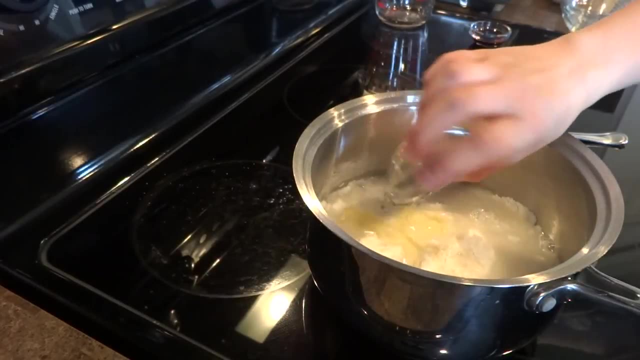 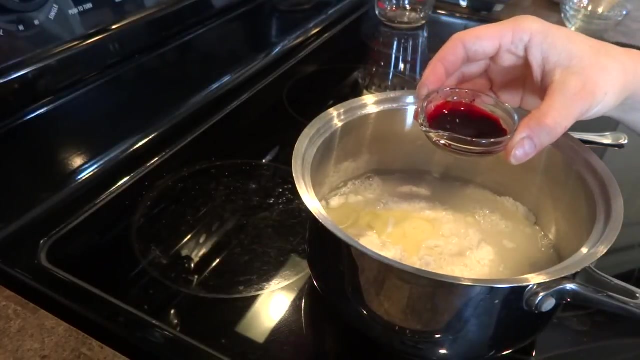 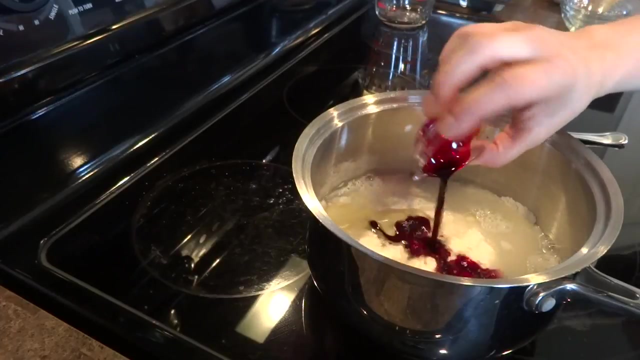 Alright, then what you need is one cup of water, one tablespoon of vegetable oil and approximately one to two tablespoons of food coloring, depending on how bright you want your play-doh color to be. Okay, I used about a teaspoon and a half. 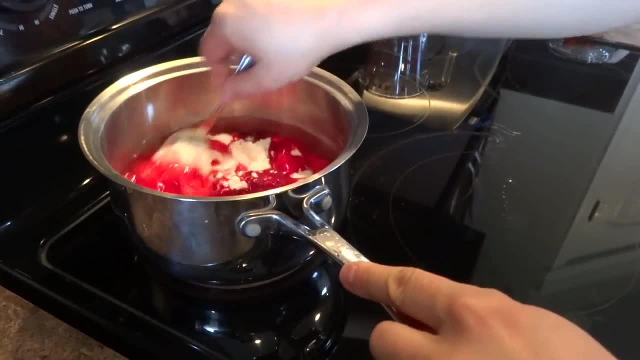 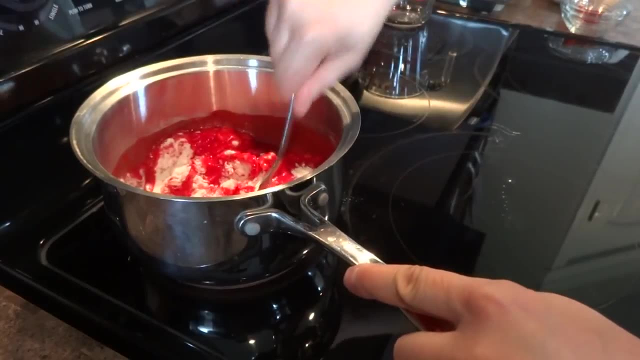 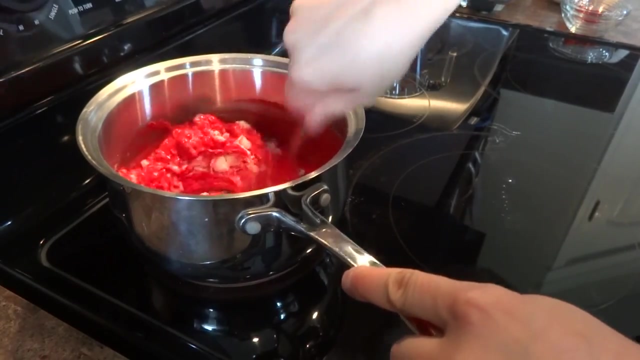 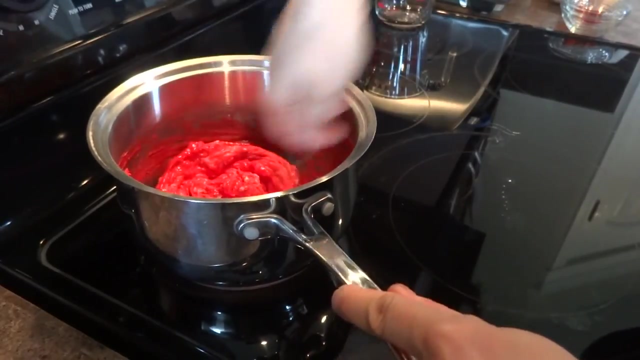 Alright. so now we're going to mix this over medium heat for maybe about five minutes. Okay, mix this over medium heat for about five minutes, Alright. so now we're going to add the flour in and a half cup of water. Now mix it all together. 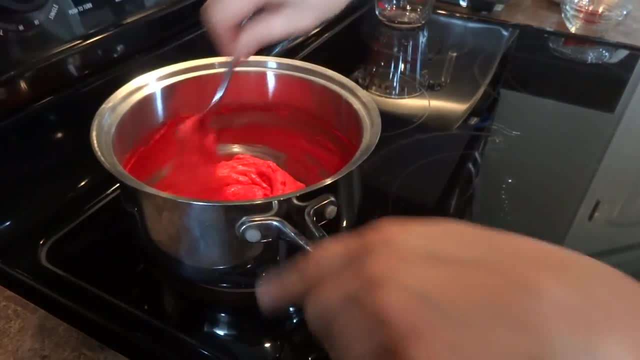 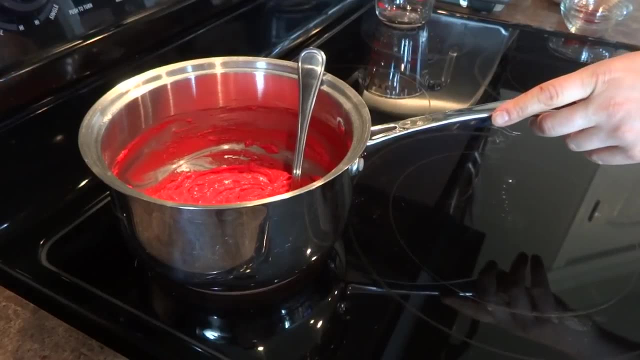 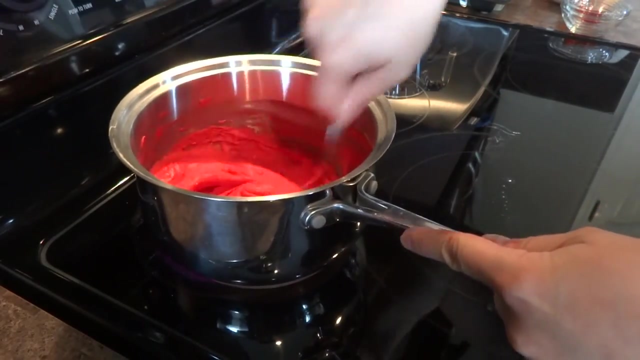 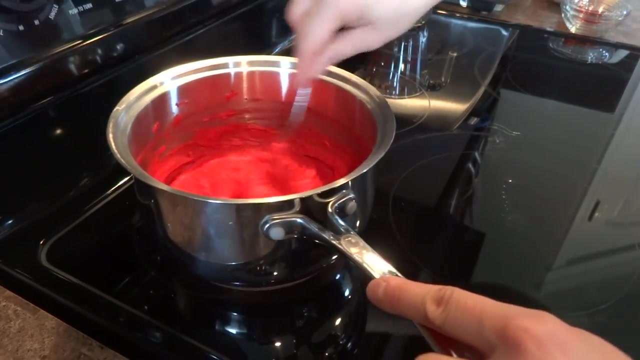 Now mix it all together. Okay, one teaspoon of salt, One teaspoon of flour, One teaspoon of vegetable oil, One teaspoon of sugar, One teaspoon of lemon juice, all right, so mixed up pretty good. I'm gonna let that sit for just a couple. 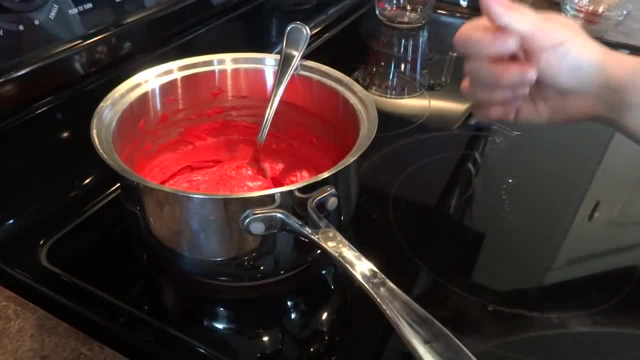 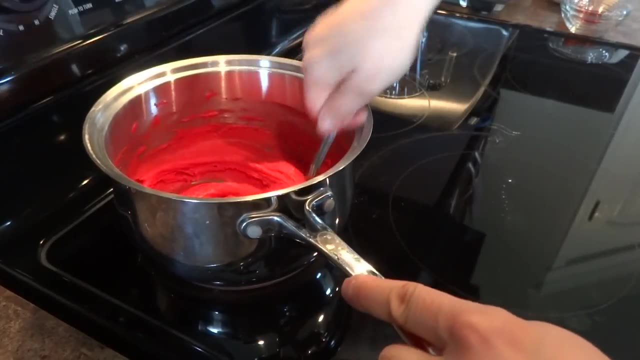 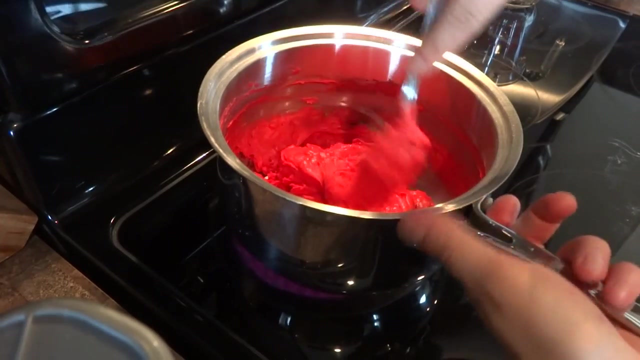 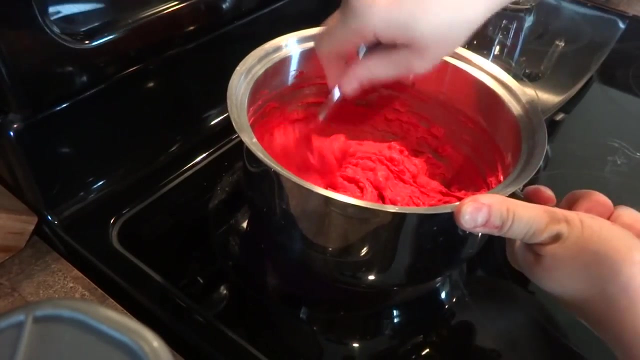 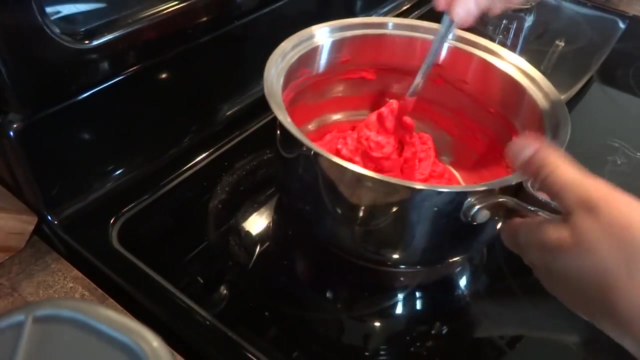 minutes here on the stove. when we get a little bit closer to ready time, I'll bring the screen back up. so just keep stirring it so it doesn't burn. all right, so my play does been sitting on the stove for a couple minutes now, all right. as you can see, it's starting to get pretty lumpy and sticky, so it's it's. 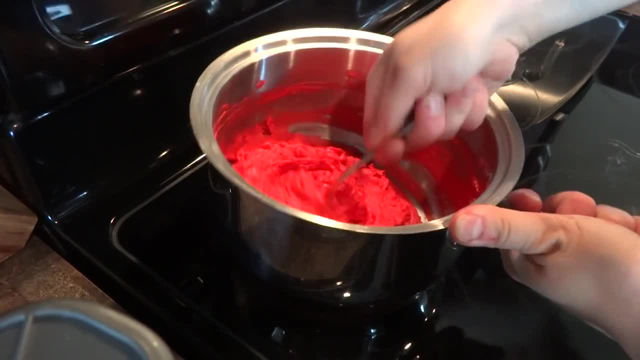 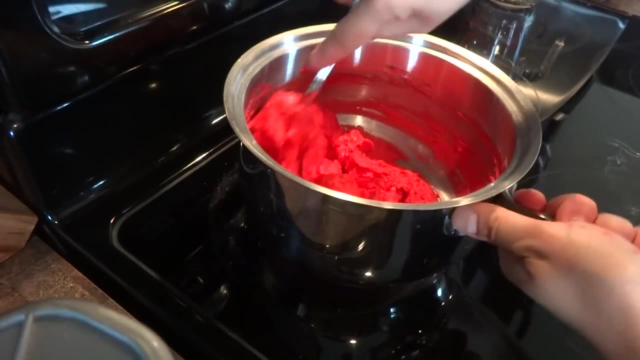 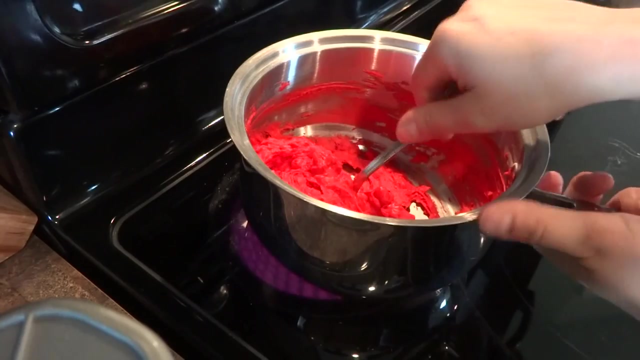 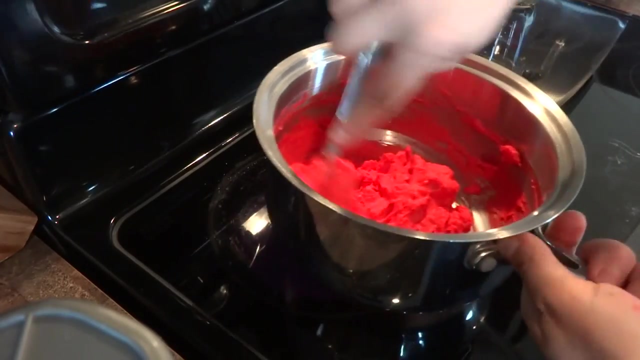 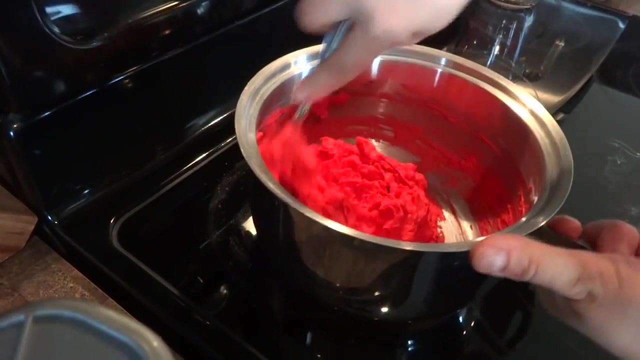 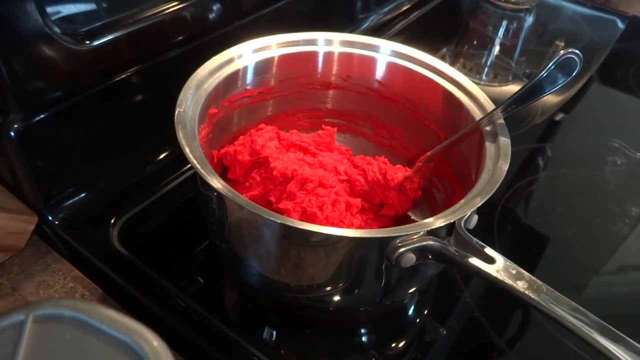 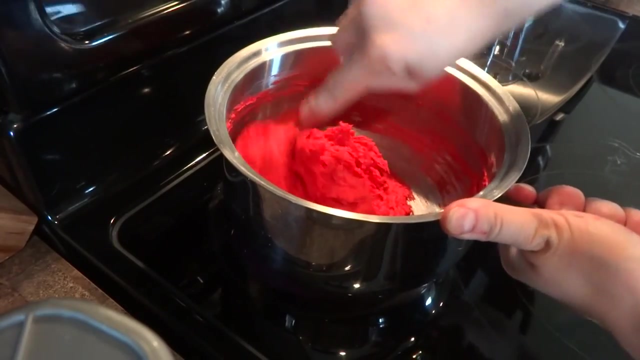 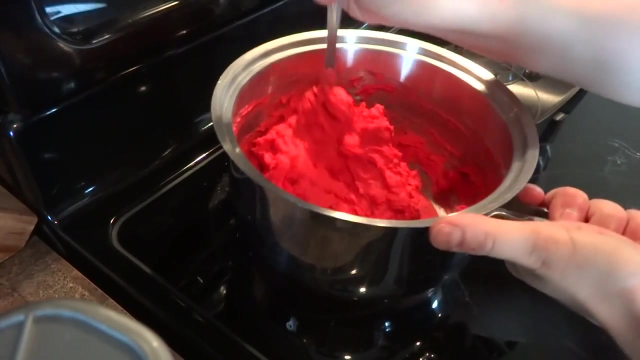 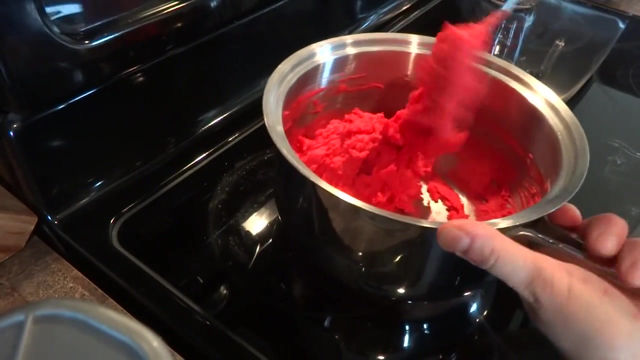 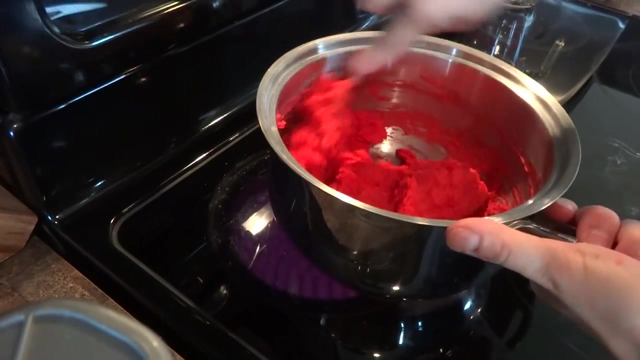 only gonna take maybe a couple minutes and it'll be done. I don't know if you can see that. see, it's getting really sticky, really lumpy. all right, come on, ruined theוף, all right. so once you've got like a great big lump in the middle of your 10. 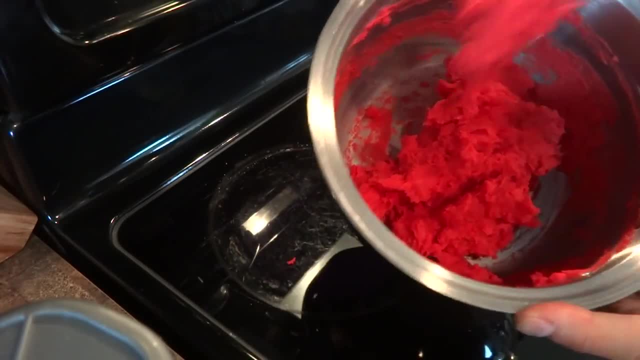 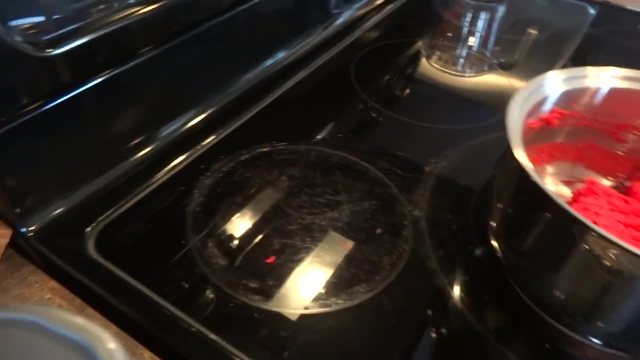 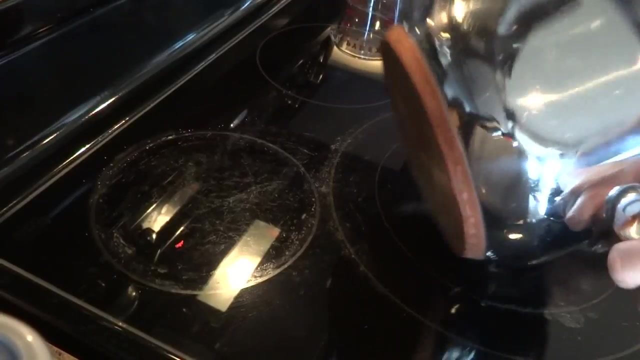 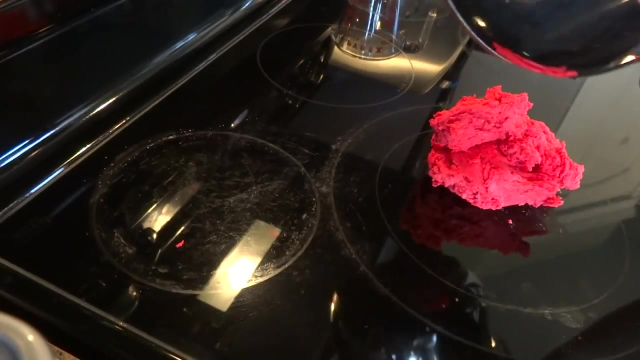 kind of like this: then you know it's ready to take out. thank you, thank you. all right, we've got our stand out ready to go. it's nearly ready to öz And start kneading, So I'm going to turn off the stove here. It's red play-doh, Emmett. 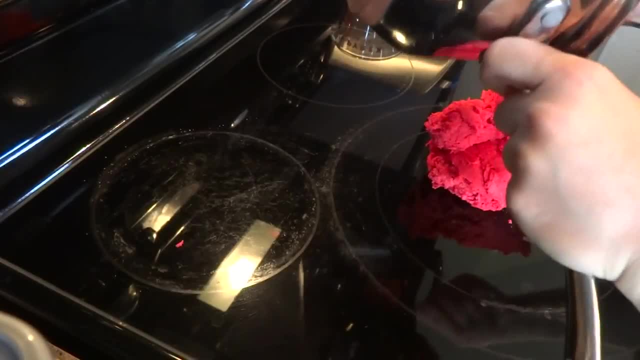 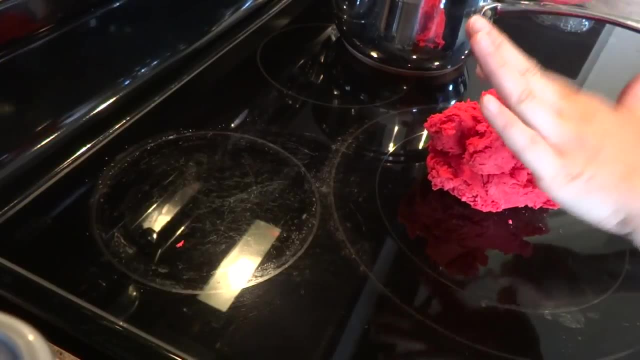 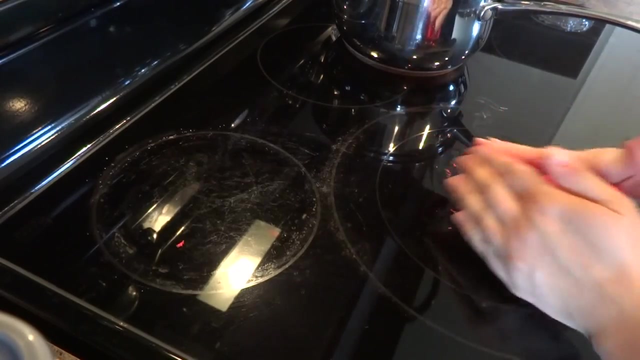 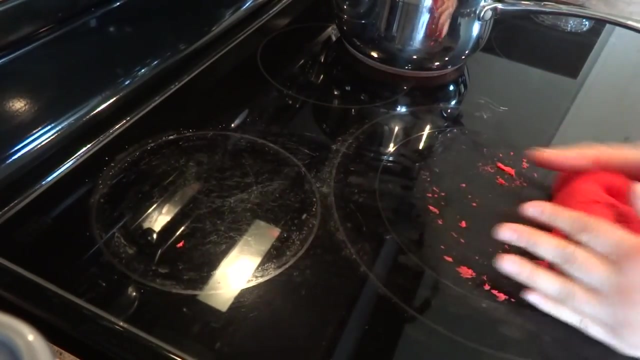 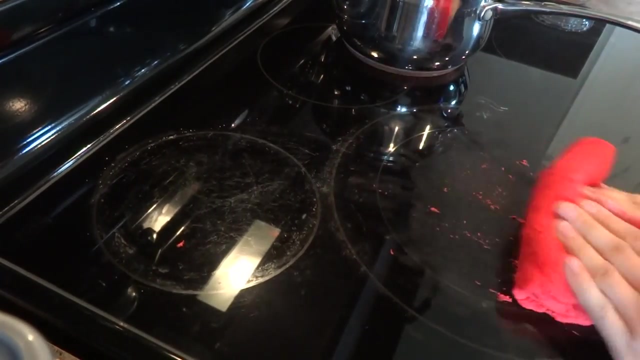 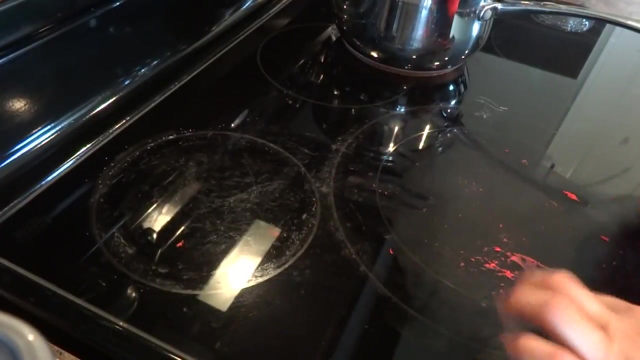 Just scrape it all out of the pan. I think it's hot, That's gooey. yes, my son says it's gooey, All right, so We're gonna just need this a little bit. Oh, You see how this one is sticking to the stove. 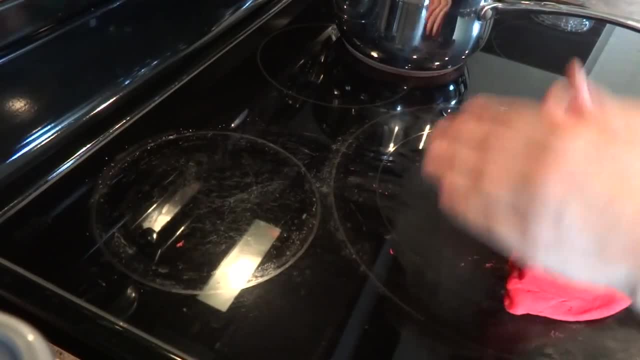 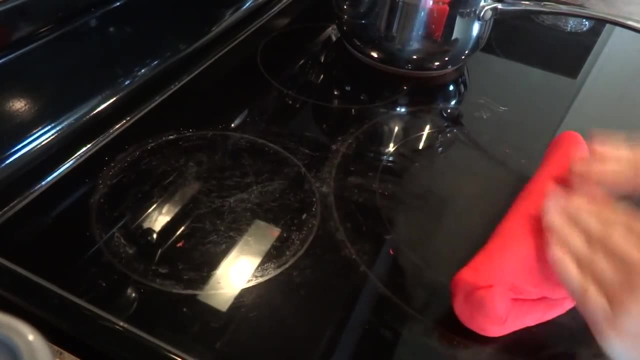 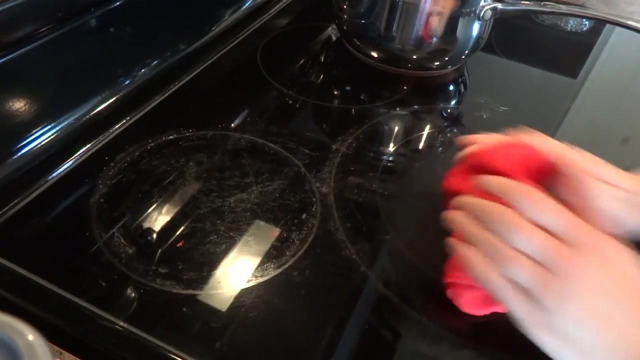 All right. So this one probably could have used another minute For cooking I made. Yeah, I took it off just a minute too soon, but if you just keep on working it it'll get better. All right, so there you go. Now you have a nice big ball of play-doh. it's ready to use.